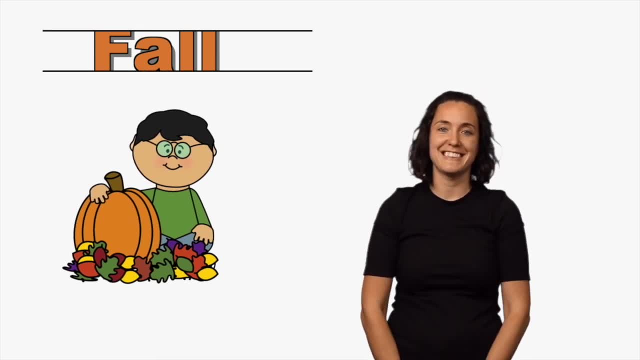 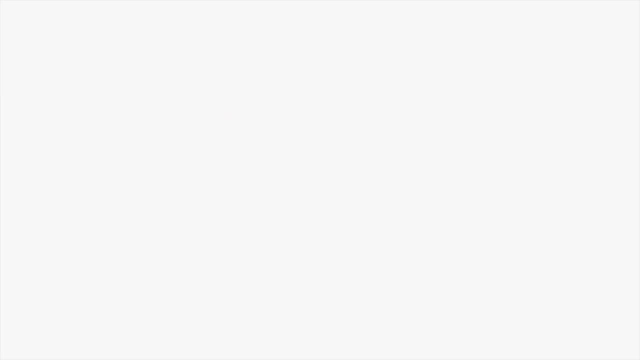 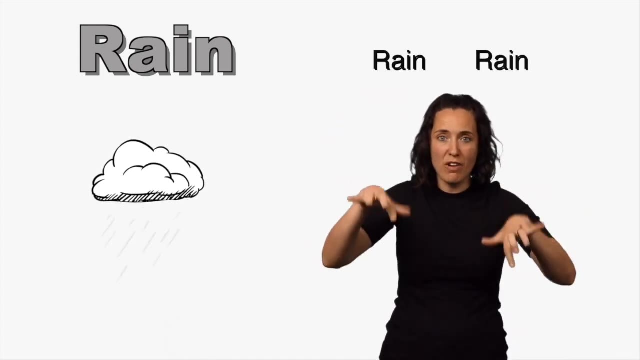 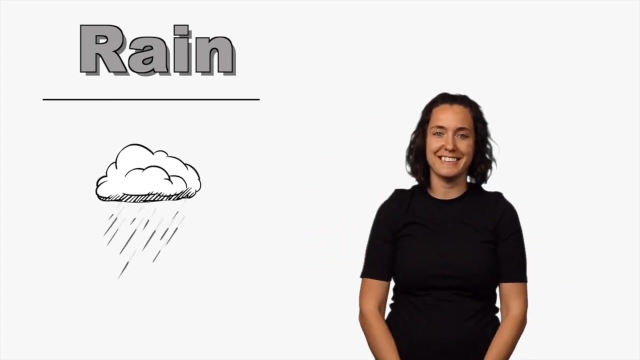 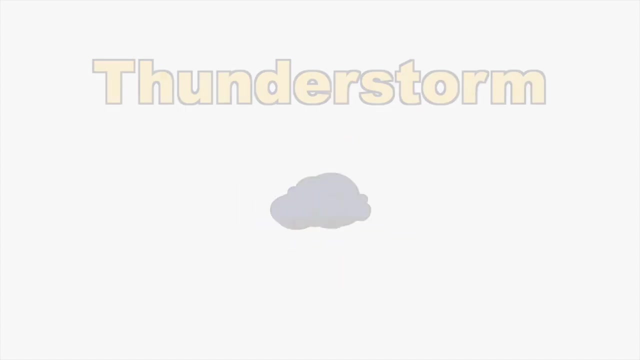 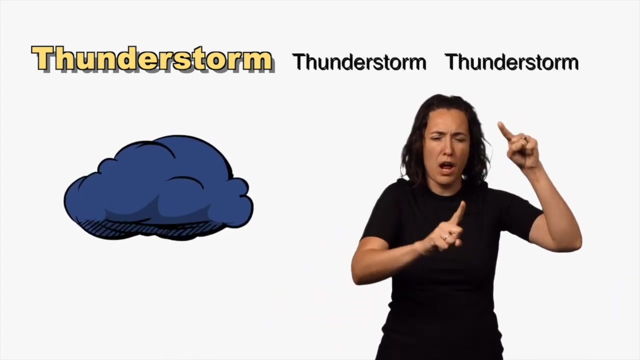 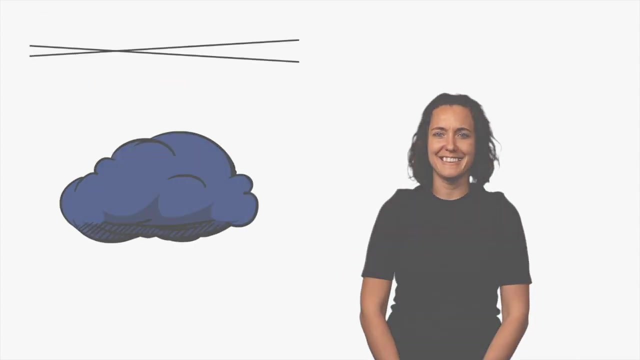 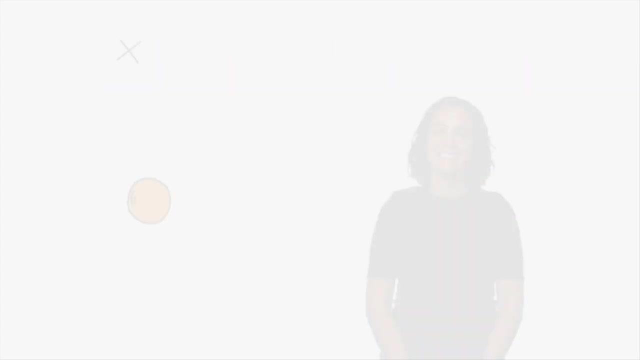 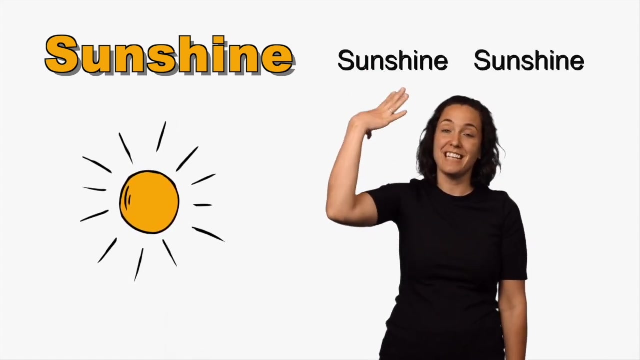 leaf- Joseph Center leaf rain, rain, rain, drip, drip, drip rain, rain, wet, wet, wet rain, rain drip, drip, drip. thunderstorm, thunderstorm, thunderstorm, loud, loud, loud thunderstorm, thunderstorm, flash flash, flash thunderstorm, thunderstorm, loud, loud, loud. sunshine, sunshine, sunshine, yellow, yellow, yellow sunshine, sunshine, hot, hot, hot sunshine. 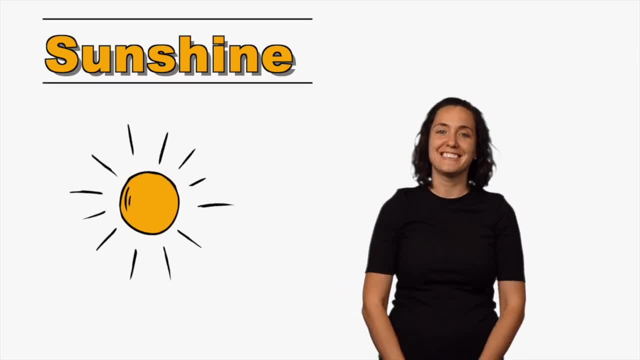 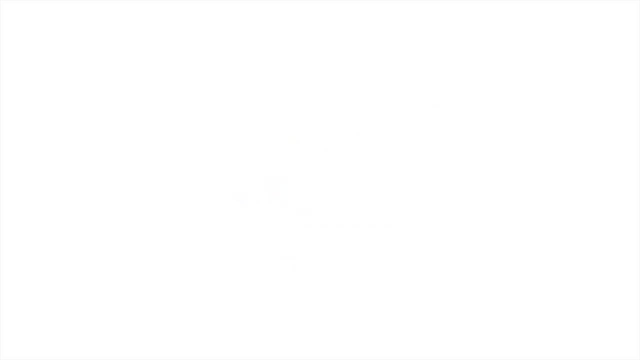 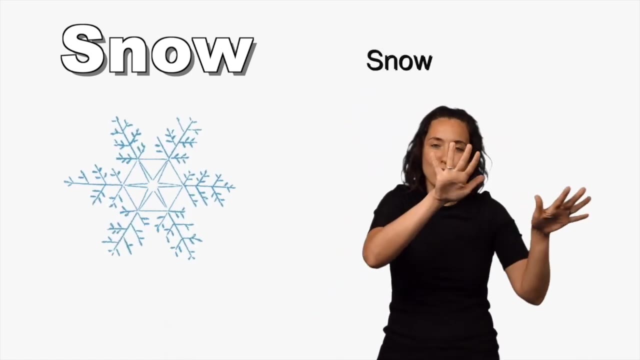 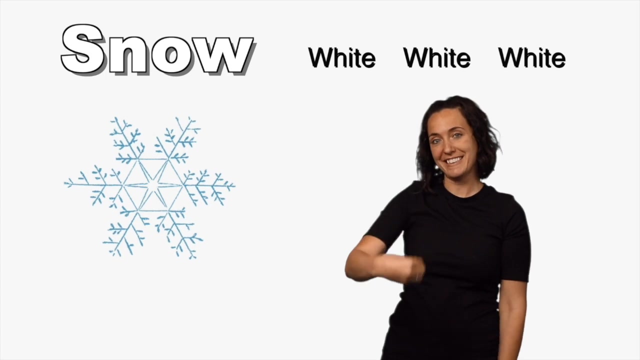 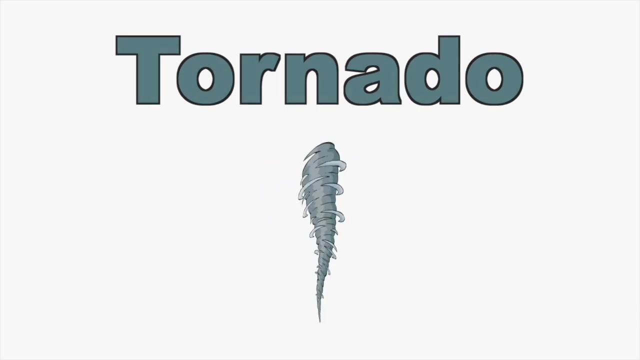 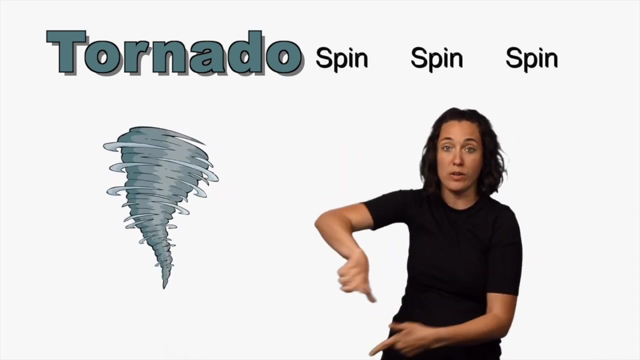 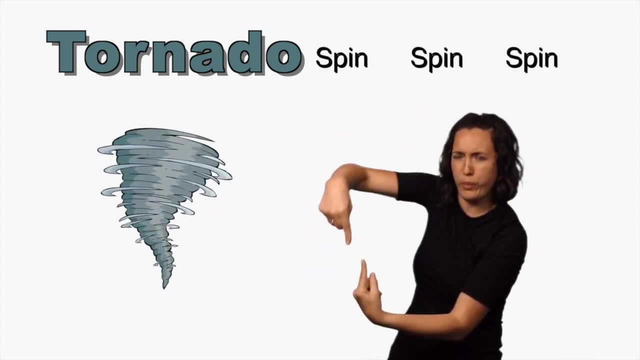 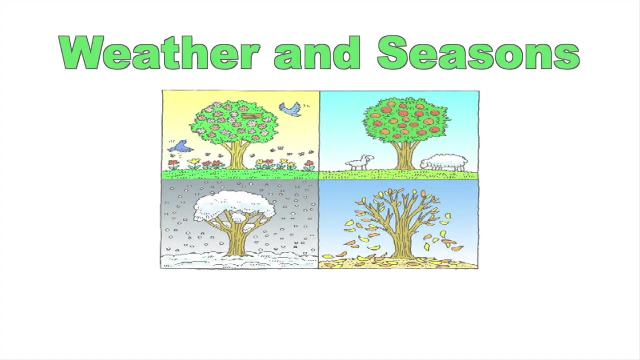 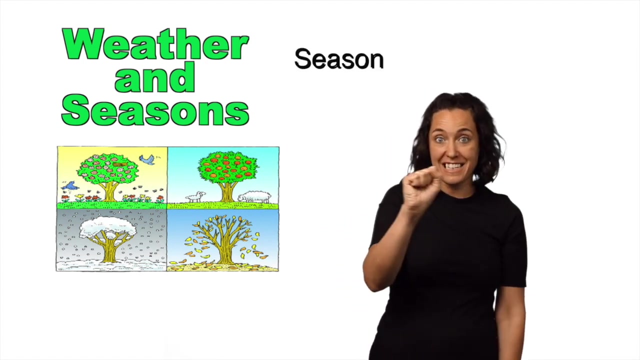 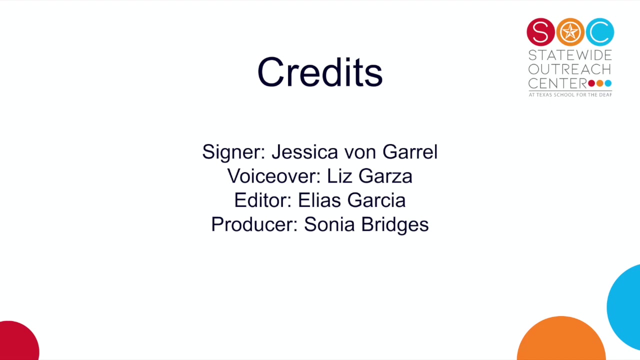